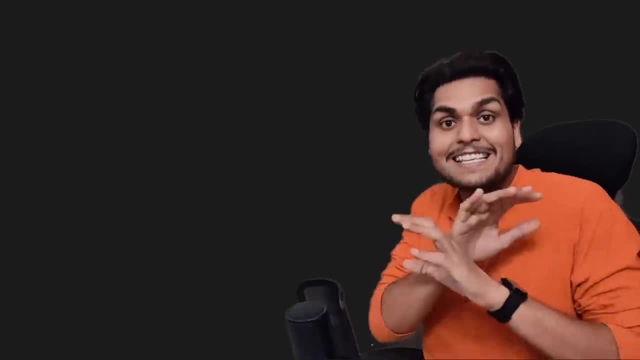 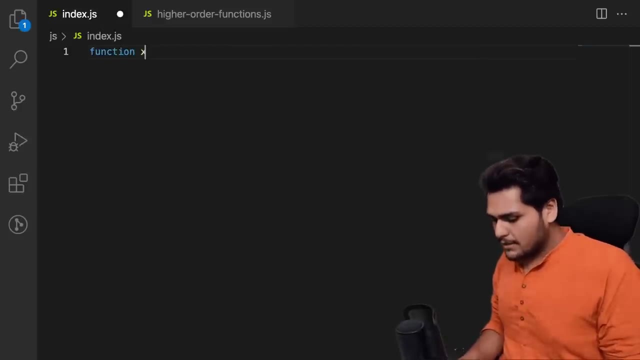 from, it is known as higher order function. Yes, it is that simple, It's that only. So let me just show you how it works. Let me just show you an example. So suppose, if you have a function X, okay, and then what we do? we just do a console log in X. 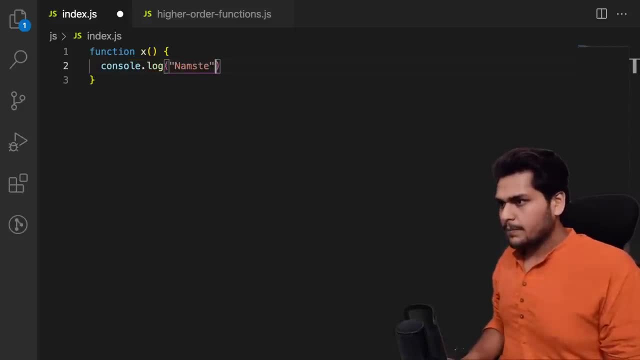 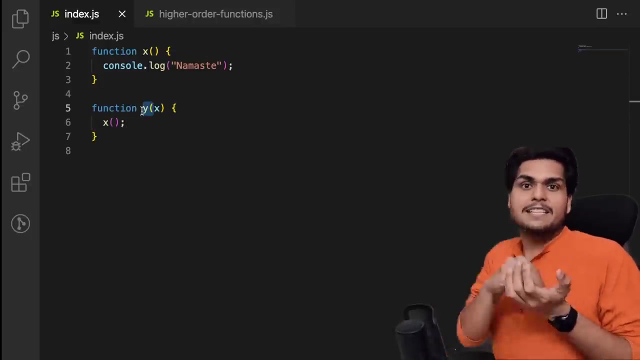 Let's do that. Um, let's call it Namaste. And we also have a function Y, which takes X as an argument and calls X. So in this case, this function Y over here, which takes another function, X, as an argument, is the higher order function. 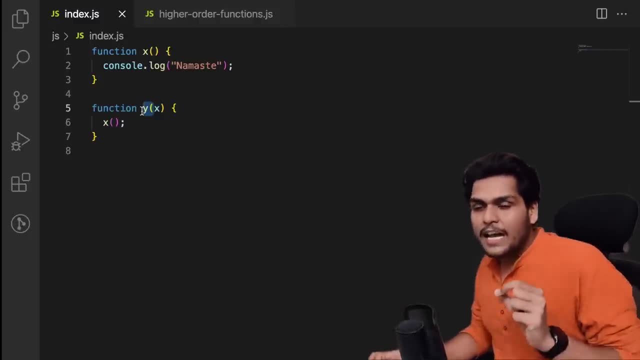 So Y over, here is the higher order function. And what is X then? So remember, remember from the previous videos. So if you're watching the previous episodes, so in the previous episode I have told you that X is the callback function. Okay, 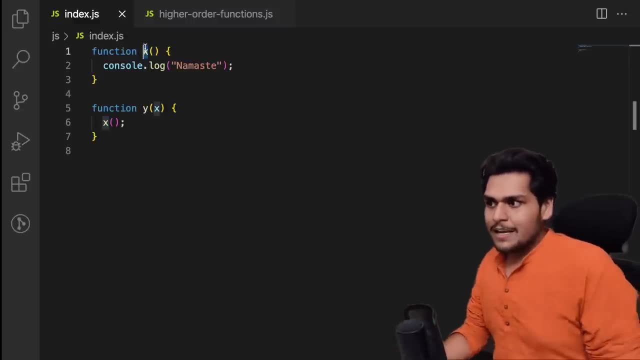 So X is the callback function and Y is the higher order function. Now is the time to take an example and show you the beauty of functional programming, the most important part, which I love, And I will also show you that, how higher order function works. 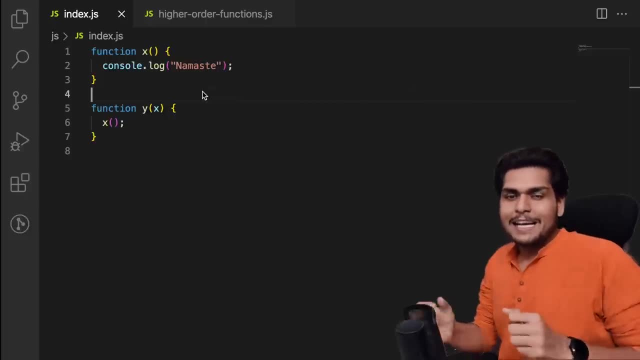 How higher order functions are very important for functional programming. Please, I request you just five minutes. Give me five minutes and keep on watching. Watch the whole example. I will show you how you should approach a problem in interviews and what mistakes do you make. Okay, So keep on watching till the end. I'll show you the example. 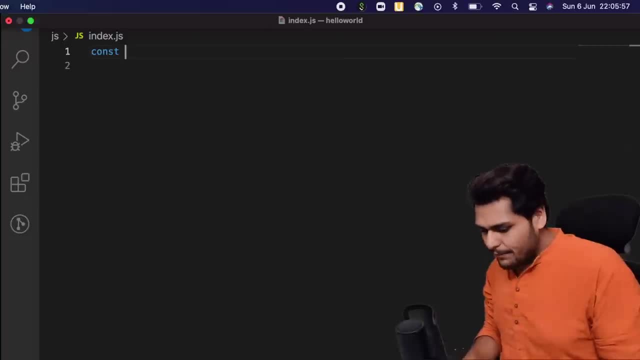 So suppose, let us take an example where we have an array which has radius of four circles. Okay, So we have an array which has radius of four circles. Let's take this as three, one, two, four. Okay, So these are the radius of four circles. 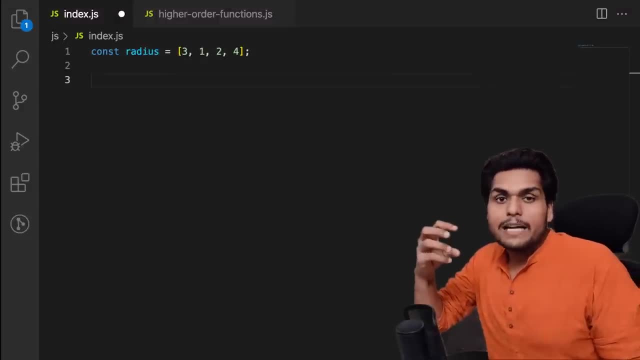 Now our task is to kind of calculate the area of all these four circles. Okay, So how do you do that? So how do you write the function to calculate the area of all these four circles? So most of us will write a function like this, right? 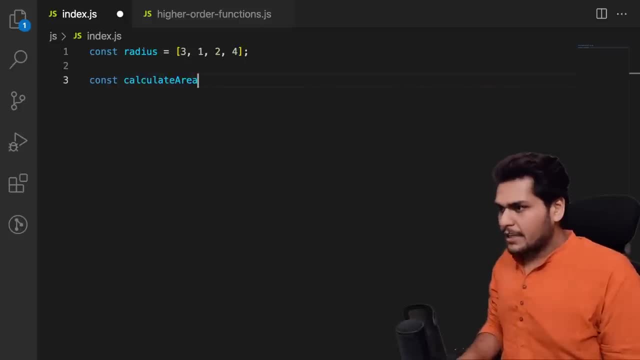 Calculate area, And then this area function takes radius as the input. Okay, So let us just say radius, And over here what we will do. we will now create another array with area in it, of these respective radiuses. Okay, So what we will do. 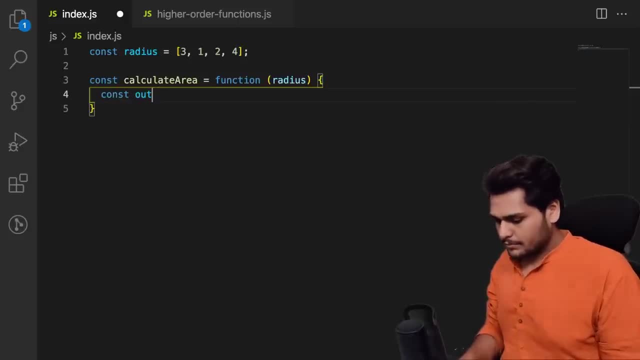 let's create a constant output And this is an empty array. And what we'll do now? we will iterate through all the radius. So let's say I is equals to zero, I is less than radius dot length, I plus plus. 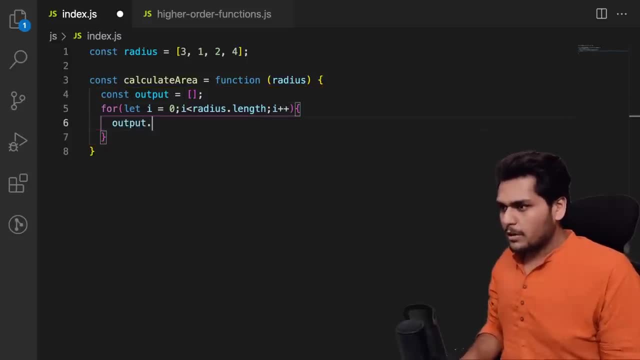 And then what we will do? we will just do our output dot push. And what will we push inside this function? It will be the formula of area, which is pi r square. So math dot pi into radius of I, into radius of I. right, This is how you'll write. 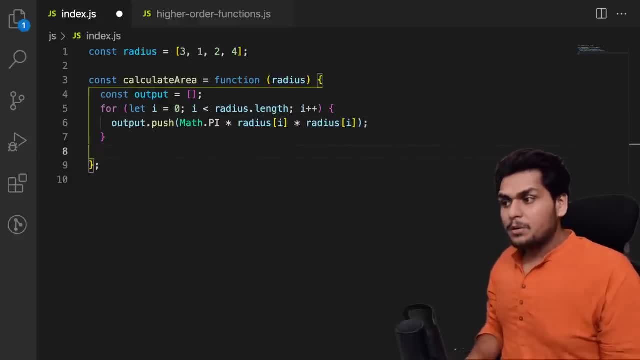 This is how most of us will write right, And then what we will do: we will just return the output. So now let us just run this function and check if it works. So we will just calculate area and pass in radius over here. 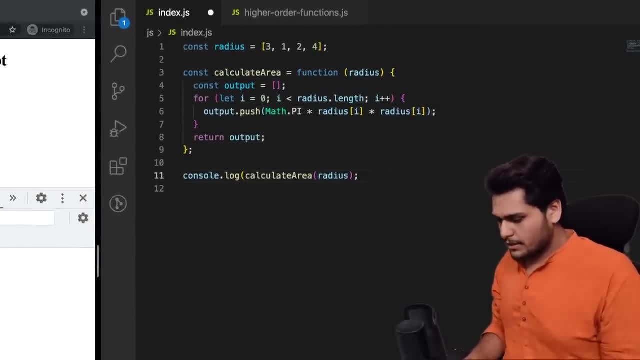 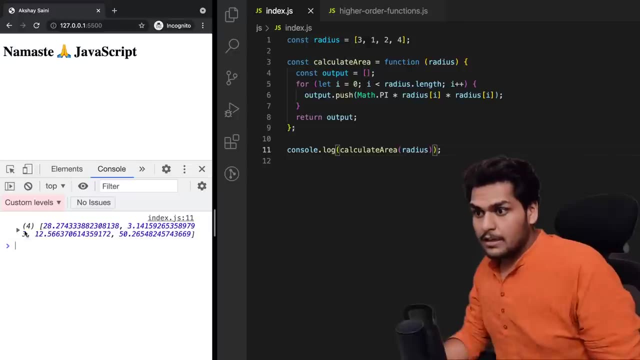 And let us log to check whether it shows us something or not. So if we run this function, so now see, this is the area, what we got. So this is the array of areas. Okay, So this is the area of four respective circles. 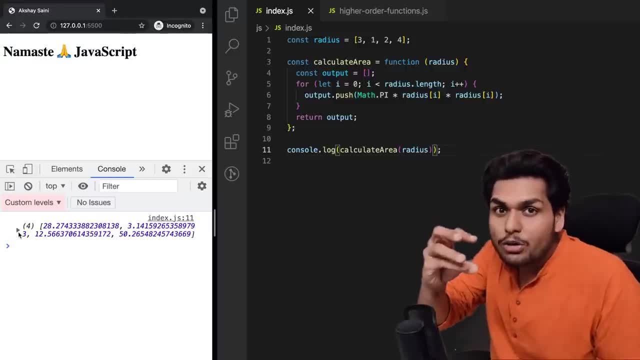 So this code is, This code is fine, This code is perfectly fine. Now I'll show you that as the code grows, what mistakes people make. Okay, So what I have observed in interviews, So what happens is suppose this time it was calculating area and this is okay to. 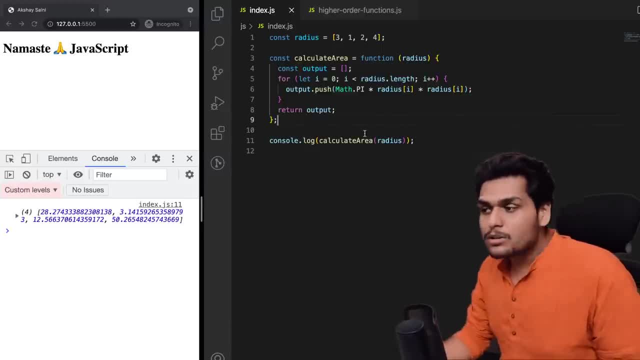 do this. but what if you had to calculate circumference of these circles with this radiuses? Okay, So what we will, what we would have done, is we then again calculate, calculate. We write a function which calculates circumference, circumference. and what we will do. 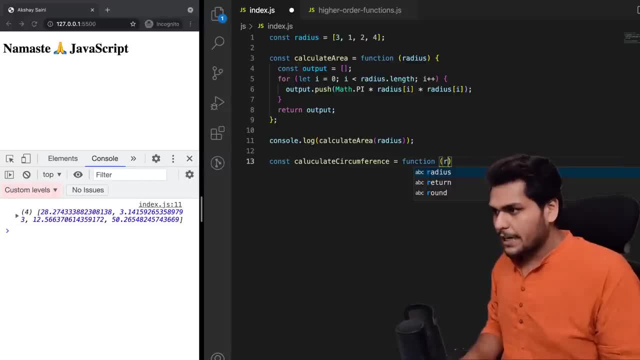 we will again create a function which will take a radius and which will do the same things again. Let me just copy it. Let me just copy this function And what we will generally do. we will just change the formula over here. So instead of PI R, square. 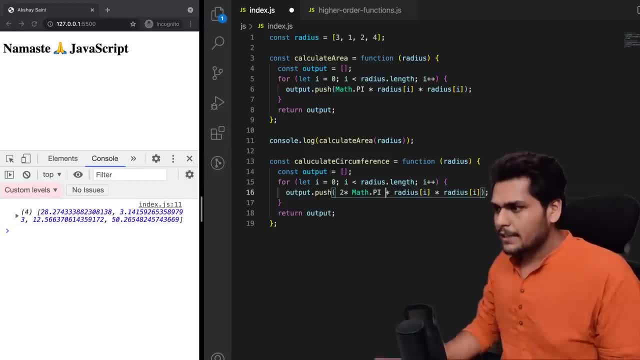 it will be two PI R, So two PI and the radius. So now let us just remove this. So this is a, this is a valid circumference right, And if we just have to print this, let us just print this circumference. 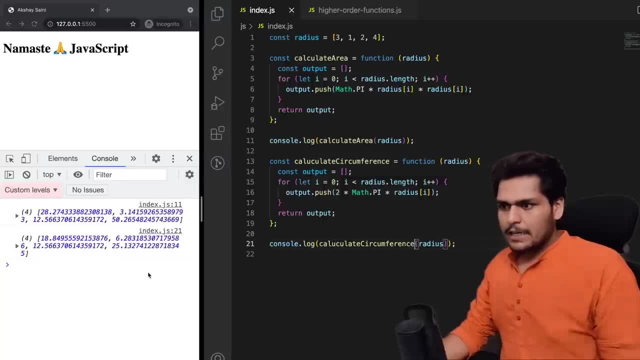 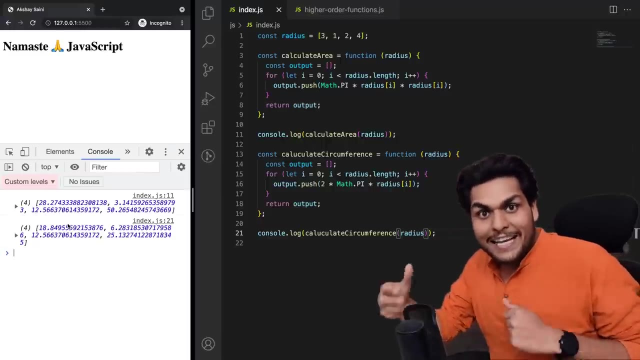 So now you can see that we have our area over here and circumference is over here, right? This is how generally people write in the interviews. and to complicate it a little more, What if you had to also calculate diameter? diameter of the circle. 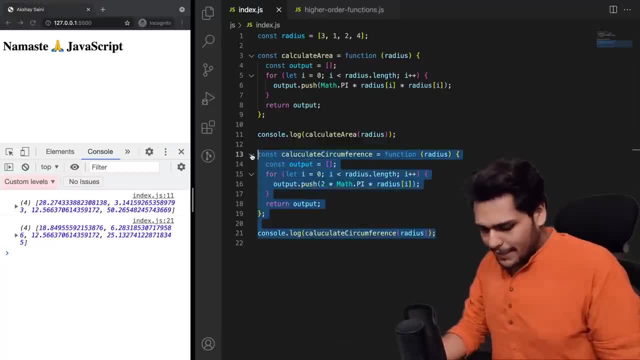 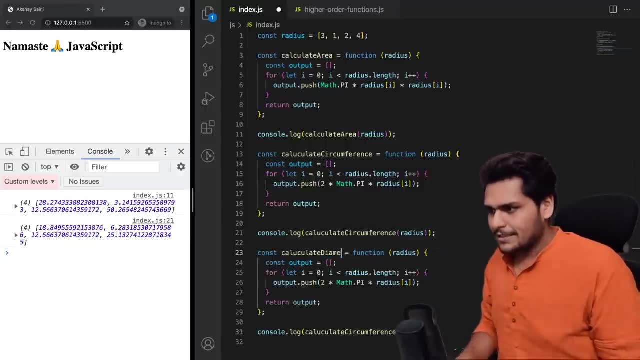 What people would have Generally done is they would have just taken this function And then generally what people do is they just copy paste it and write it like this diameter, And what they will do change the formula of the function over here And we will have our diameter function ready for. 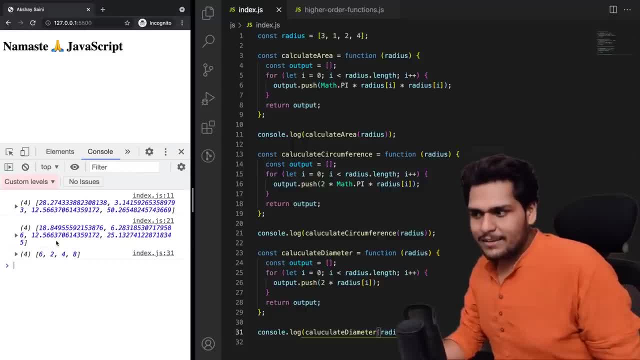 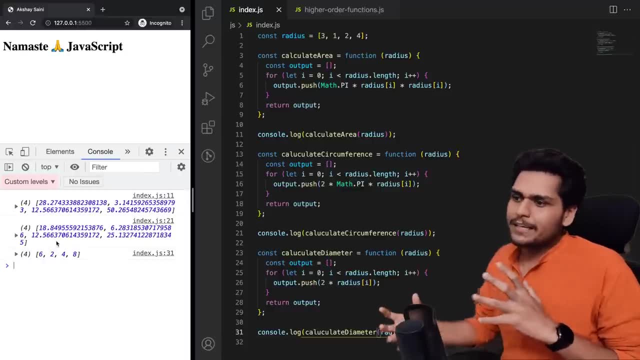 us And this will now print the diameters. So this is how, generally, I have seen a lot of people hurrying and copy pasting and doing code, but this is not a good way. Do you see a problem here? Can you see a problem here? 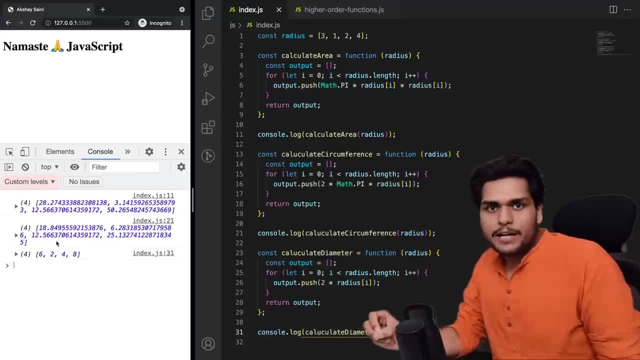 I would like to give you a moment and think: what is the problem over here? Can you identify a problem? And if you identify, we will try to solve it And I'll show you that how you should write the code. Okay, I will show you what the interviewer expects you in a coding round. 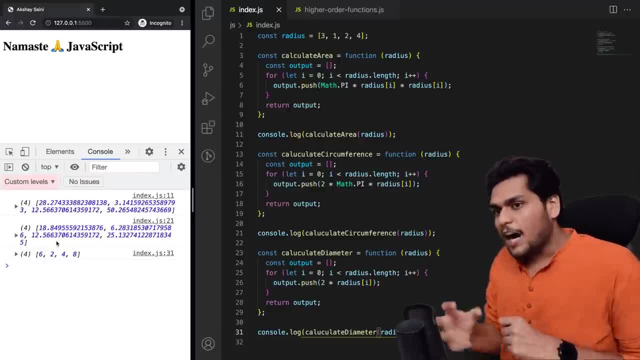 What is modular code, What is reusable code, How you can write it in a functional way. Okay, So first of all, let us see what are the problems over here. The first problem, which you can obviously see- and you would have hit off- is that we are repeating ourselves a lot. 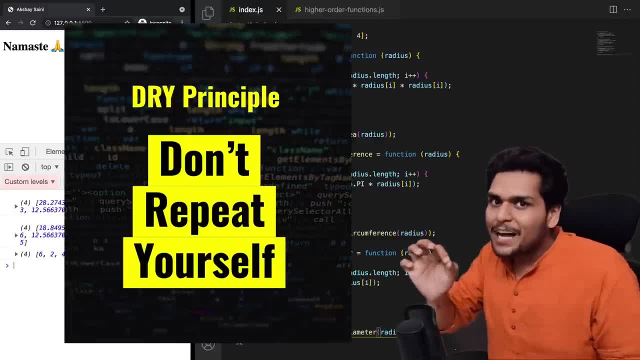 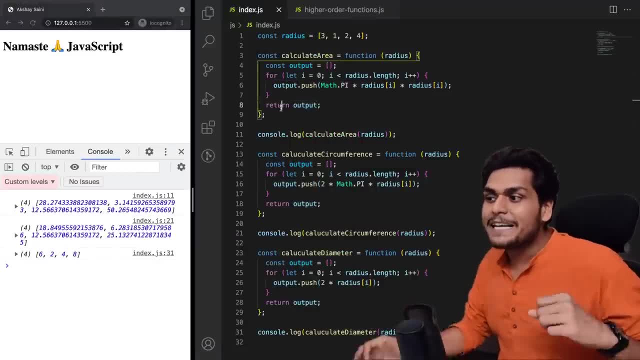 So there is a principle in software engineering which is known as DRY principle. DRY principle, which is: don't repeat yourself. So over here, what we see is generally we are repeating ourselves a lot. All these three functions have almost 90% of the code. 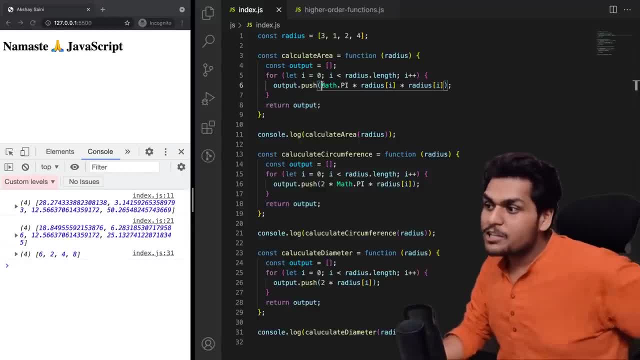 which means the code is the same, isn't it? And what changes is just this logic, a logic of area, a logic of circumference, a logic of diameter or maybe something else? The only thing changing is that logic. So can we write it in an optimized way? 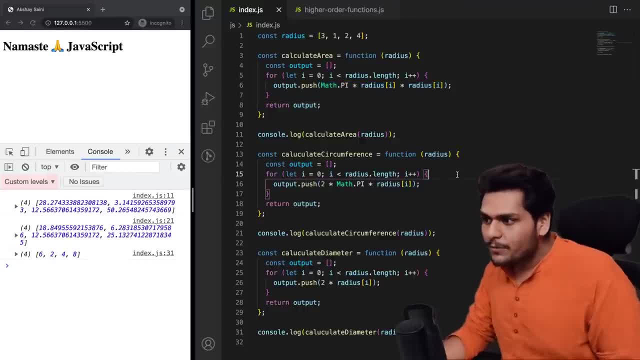 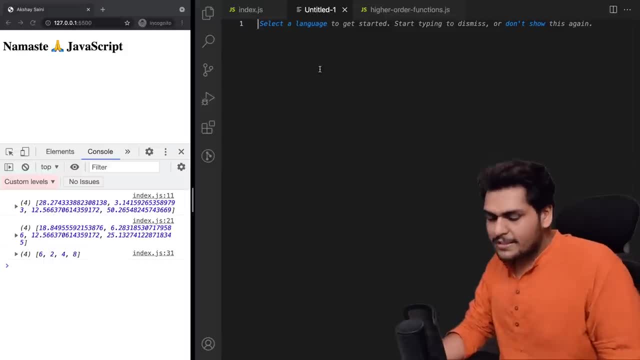 Can we write it in a better way? Let's see how to write that. First of all, I will be making changes, So let me just copy and just put it in the new tab, Just for reference. we will just compare it later on. 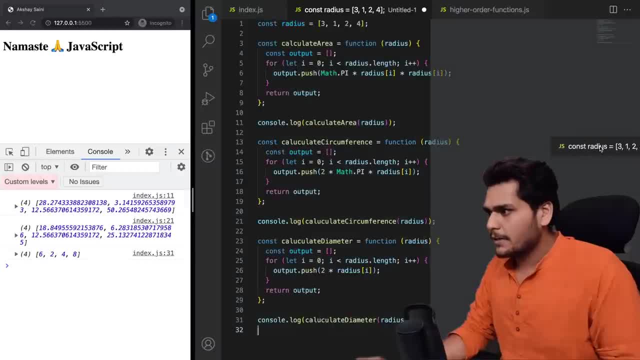 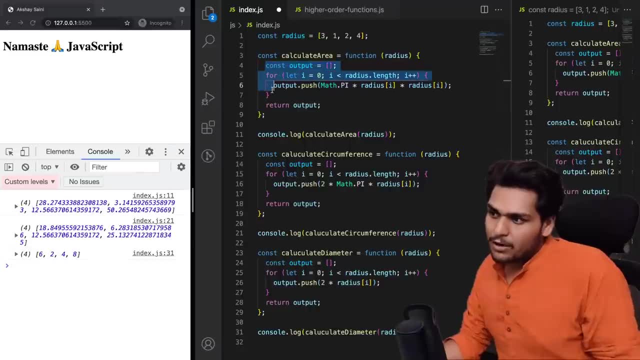 Okay, And let me just move it aside over here for the time being. Okay, Now let us just try to optimize our code. So see, we are repeating ourselves a lot. We are just creating this array again and again in each of these functions. 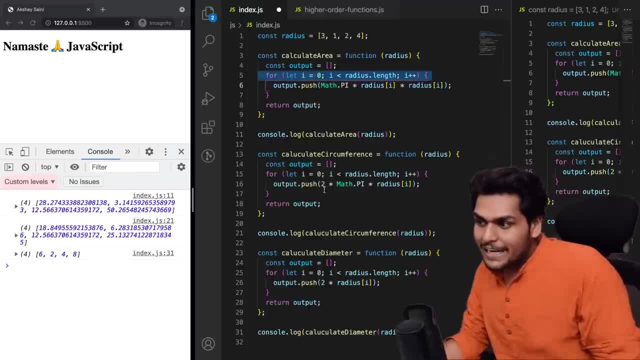 And we are also iterating through this whole statement again and again and then pushing something into the output and then returning the output And the only thing changes is the logic. So first of all, can we just abstract this logic out, Can we just abstract this logic of the area outside calculating the area? 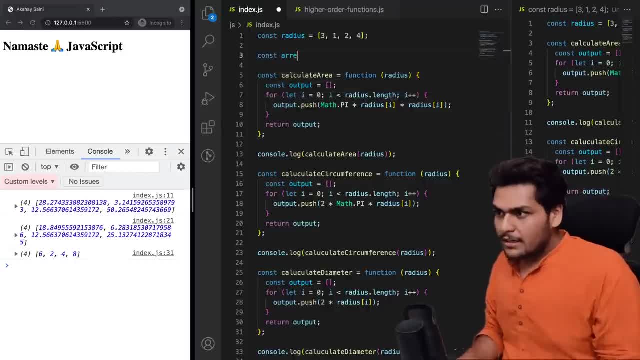 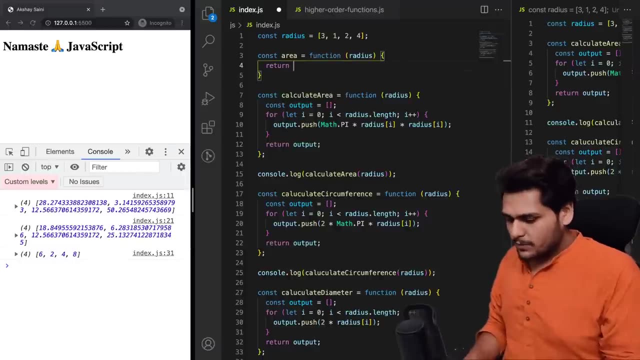 Yes, we can. How we can do that. Let's create a good way to approach. This is to create another function, Okay, Which is area, And the only responsibility of this function is to take the radius and return the area of this function. 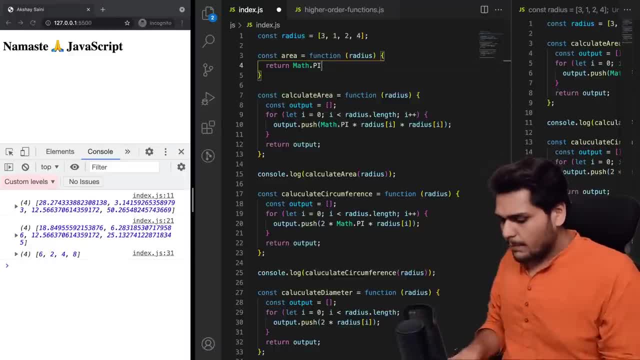 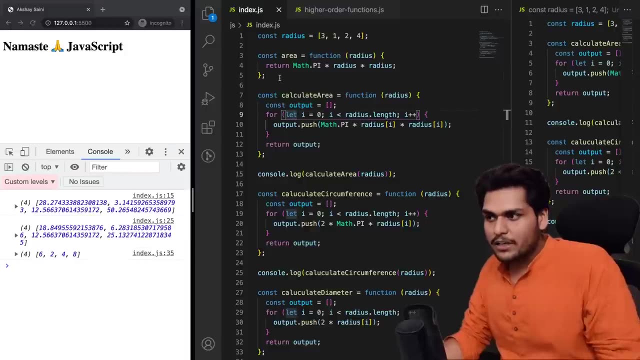 Okay, And then what we will do: matpy and then radius into radius. Okay, This is how we write a function of area, isn't it? So now what we will do, we will try to make this function generic. We will try to make a generic function and we will try to put this logic inside the function from outside. 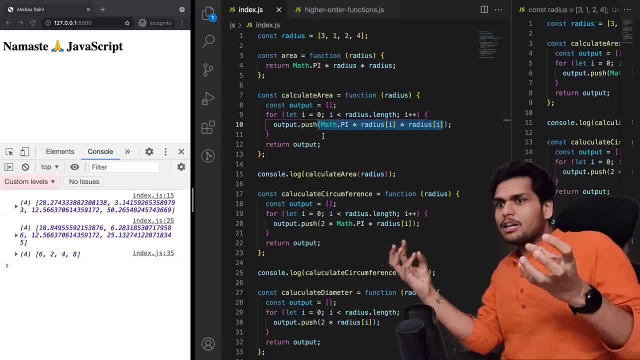 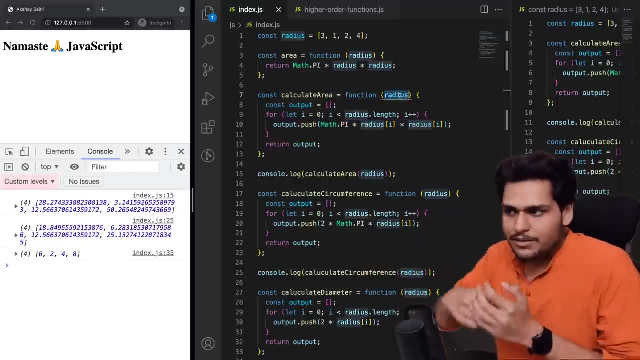 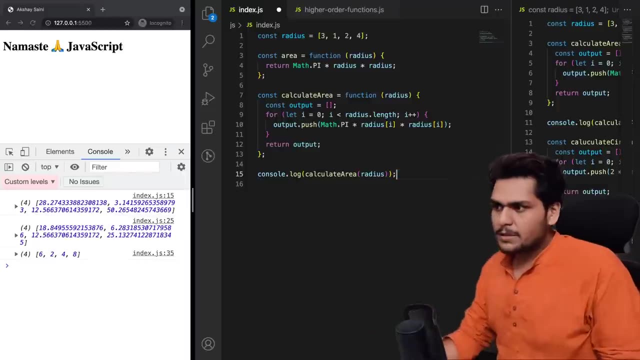 Now, this will be sounding complex, right? So kind of like: just like we are passing radius inside this function, we will be passing some logic inside that function. So it sounds interesting, isn't it? So this looks a little messy. Let us just remove all these unnecessary code and just take this area as the reference. 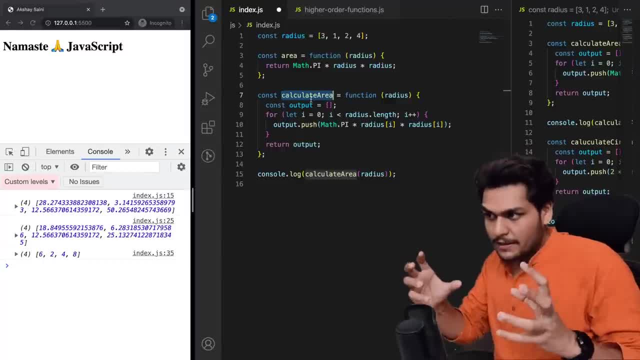 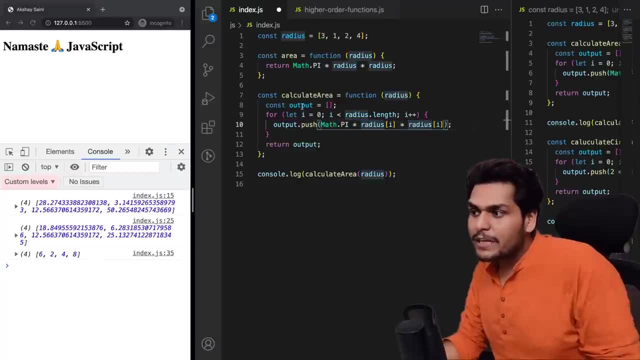 So now what we are going to do is let us write a generic function, generic function where you pass in this logic of area inside that function. That function will be very much similar to this calculate area. So let us just try to write this: 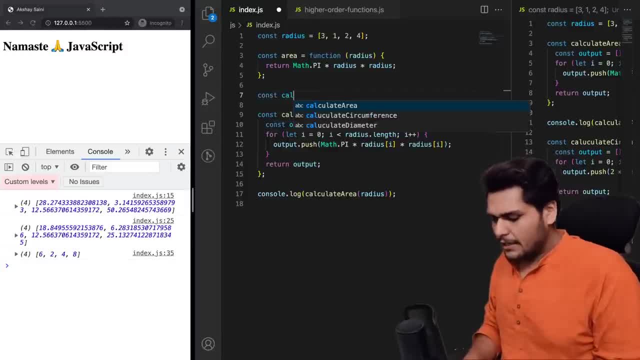 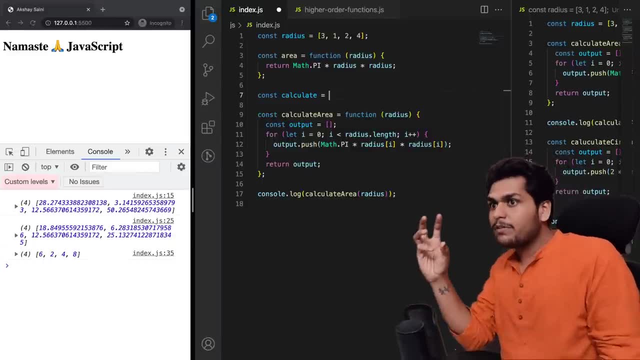 So let's name this function as just calculate, calculate and not calculate area or calculate circumference or calculate diameter. But we will pass that logic inside that function and it will be doing a similar job. So let us just copy this. So now carefully see what I am doing. 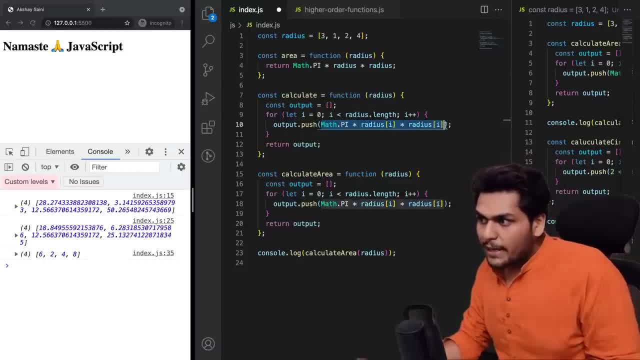 Okay so, now this logic shouldn't be written over here, This should be passed from outside into this function. Okay so, and this logic could be anything. This logic could be calculating area. This logic could be calculating circumference. This logic could be calculating diameter. 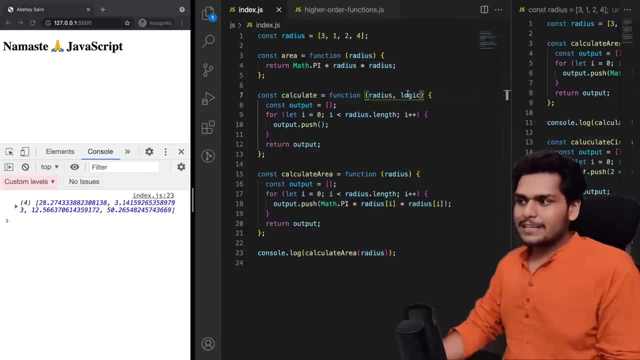 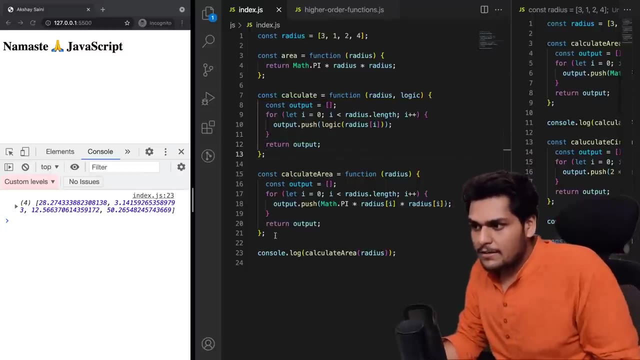 So we will kind of try to pass in a logic inside this function and what we will do, we will call this logic with radius of IE. make sense. Now it might be sounding a little complicated. Just check it once again. See this function and see this function. 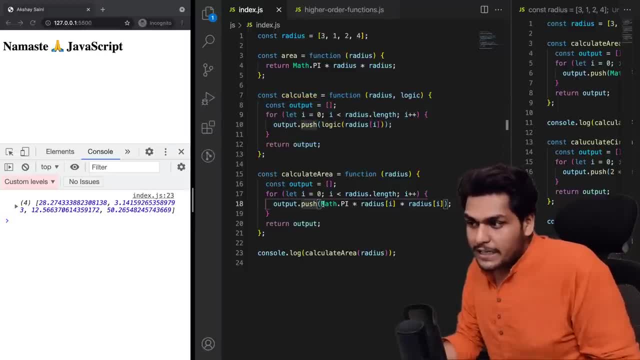 They are almost similar. What we are doing is over here instead of writing directly over here, instead of writing the formula of area directly. I am just abstracting out things. Okay, I am just passing logic inside this function and doing something. So now what I will do is just like we called this: calculate area. 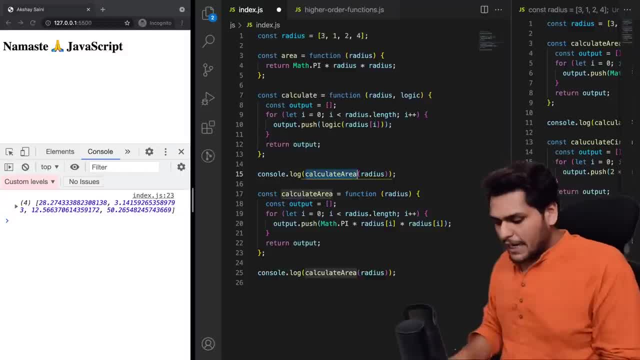 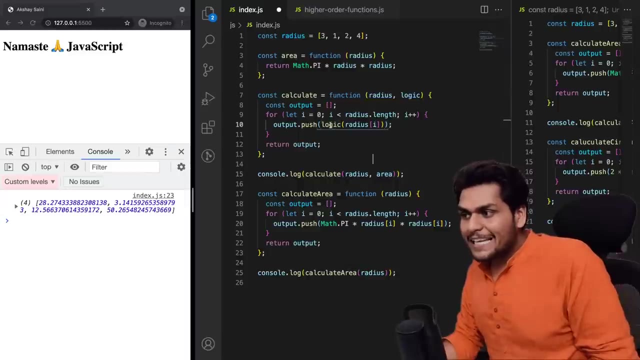 Let us just call this also calculate and in, and we will call calculate and now we will pass radius and along with that we will pass the logic to be implemented. So over here, if you see, we pass in area as the logic and now this area function will be called with this radius, again and again, for each and every element in this radius, and it will be pushed inside the output. 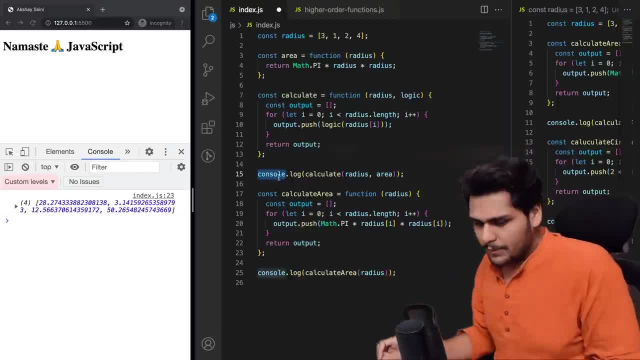 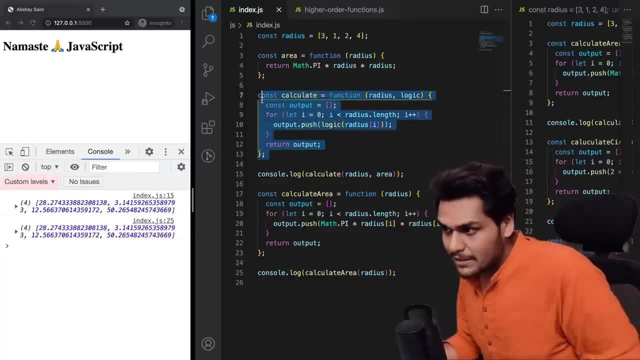 If I log that, guess what will? the output will be: So see, so the output will be same. So it is just like writing this code, but we have abstracted these things out. So now you will ask me, Akshay, that this was good code. 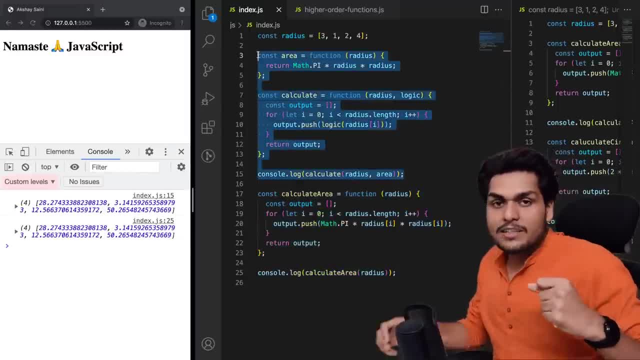 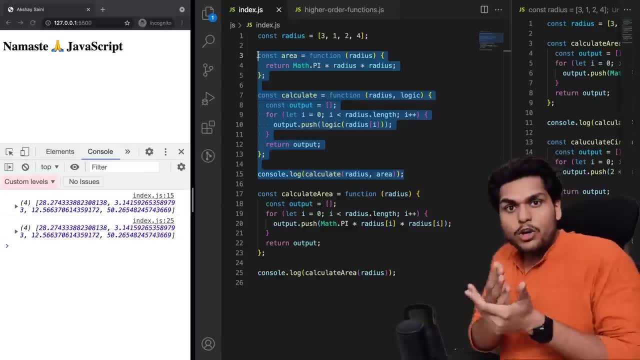 Why did you even abstracted this logic out? What is the use and why did we do this? Why did we abstracted this area out? Is it really required? But now you will see the beauty of it. Okay, because suppose if we had to calculate circumference now. 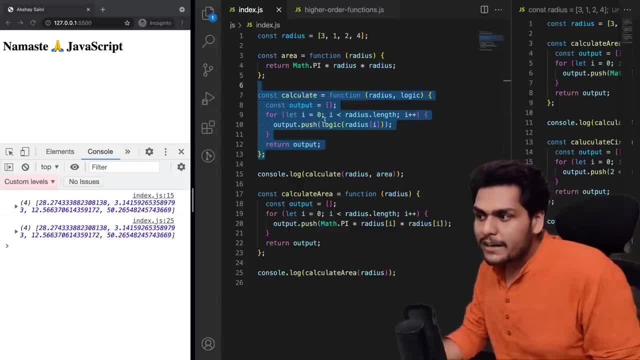 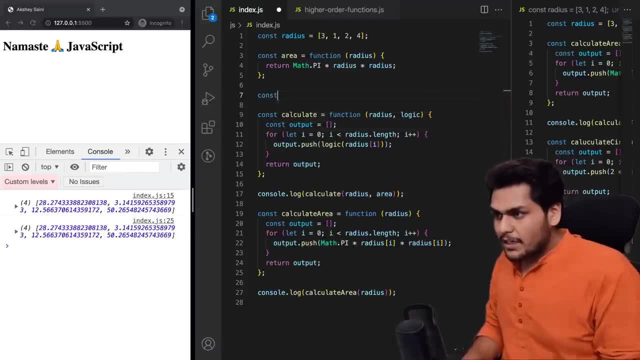 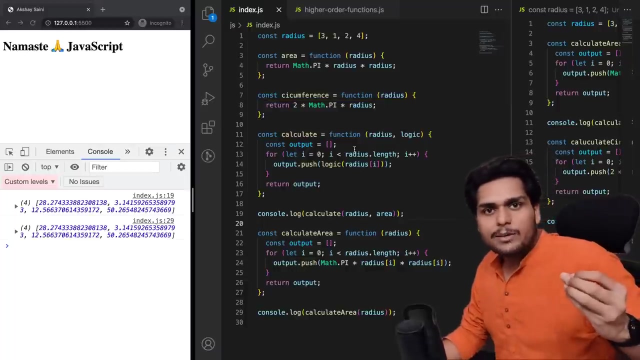 so we no longer need to copy this whole code and write the logic again. but we can just do a small thing. We can just write the circumference logic In a function over here, just like our area, matpi. So now if we had to calculate the circumferences of these circles? 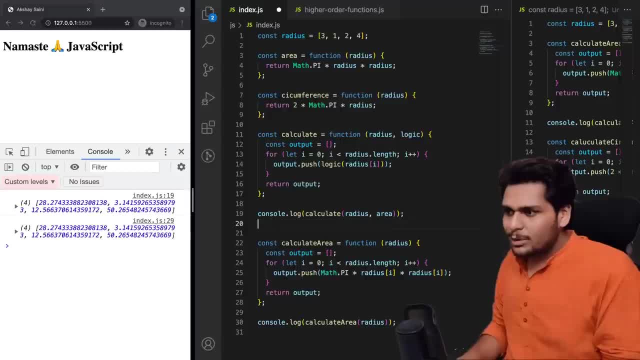 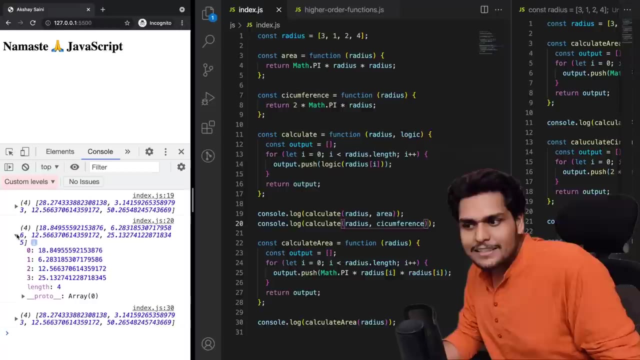 all we have to do is pass another logic into this function calculate. right, We can reuse this function calculate and just pass in a different logic over here, which is circumference. See, we got the circumference over here as output. See this: this is circumference. 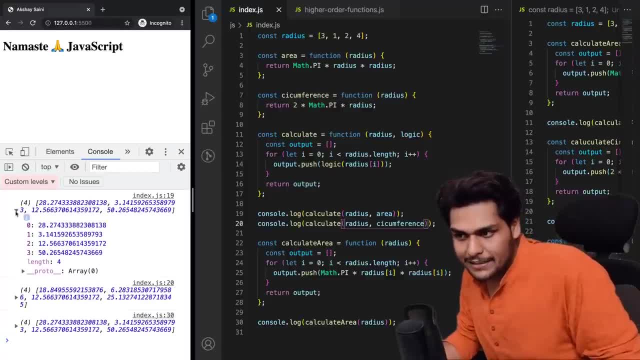 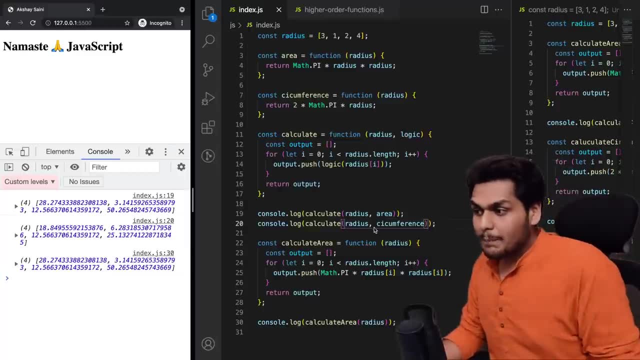 This is area and this is how we can write it, Instead of copy pasting this whole code. We have abstracted this logic out. And what if we had to pass write code for diameter. Okay, we had to calculate code for diameter. 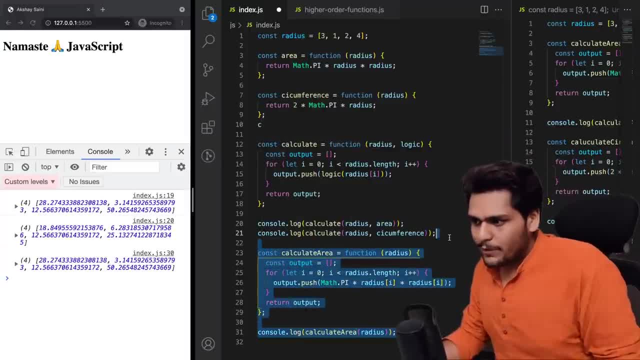 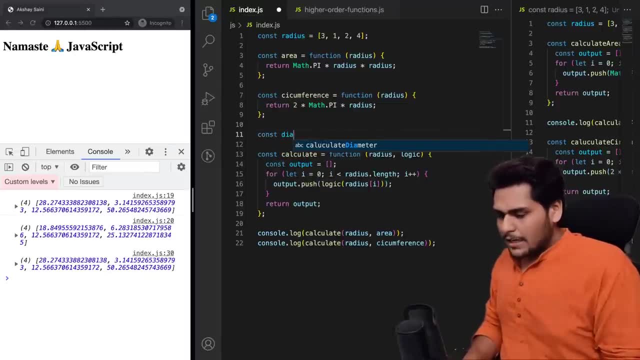 So let me just get rid of this calculate area round, So we don't no longer need it. So if we had to calculate diameter, so what we could have done is diameter and again the same thing. We just have to add in another logic over here and we need to just return. 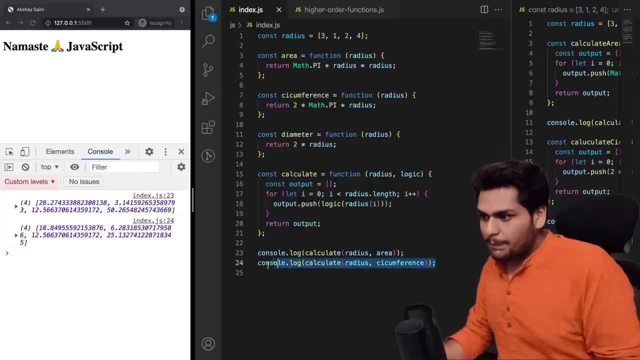 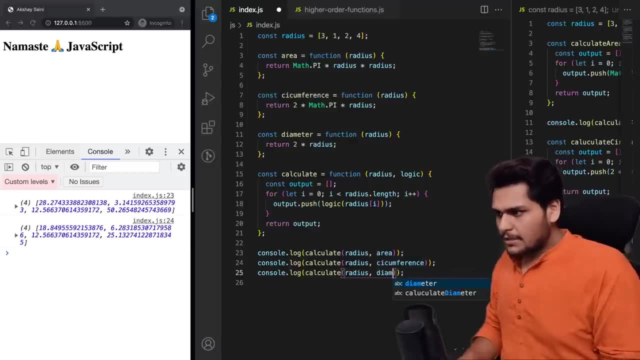 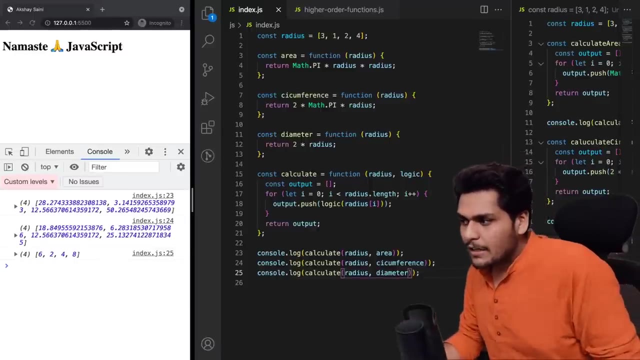 Two into radius, and we can just pass in another logic, which is diameter, and it will return us the diameter of these circles. So this is how that whole code now you can compare. So the earlier code was this and now our code is like this: 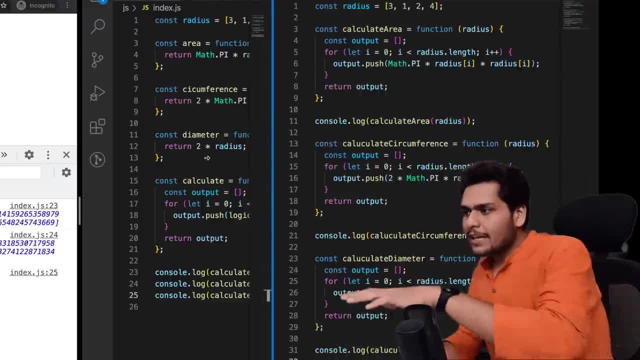 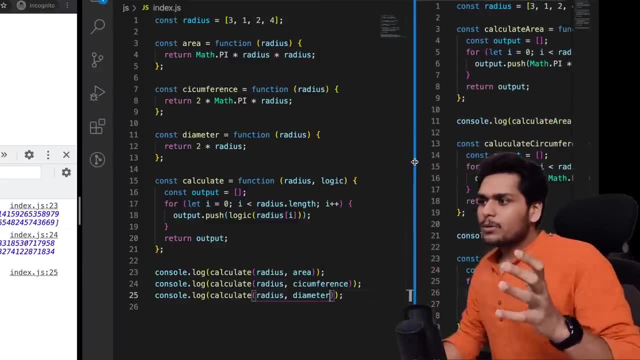 So we had separate functions for each of these logics. So in the right hand side you can see this was the earlier code and this is the new code. So now I'll tell you that why this code is good, And this is the beauty of functional programming. 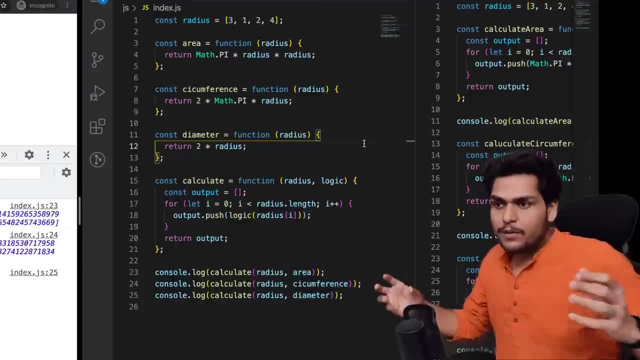 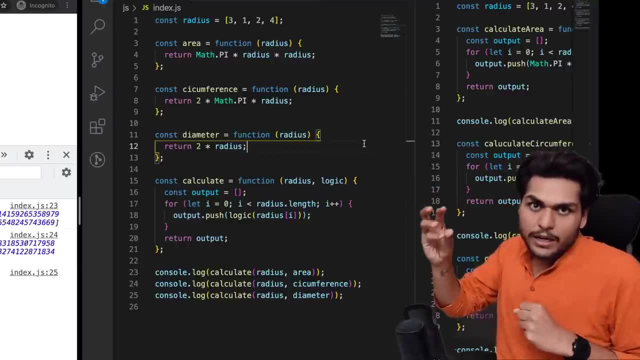 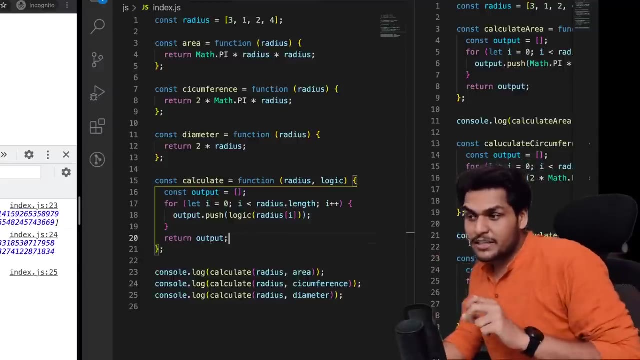 Okay so functional programming is huge in itself, but a small part of it says that think or make the logic in your head according to functions. Okay so whenever you are giving a coding round interview, then you should write your code in this fashion and not this fashion. 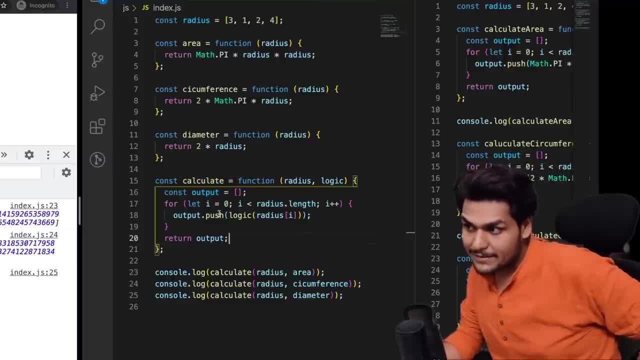 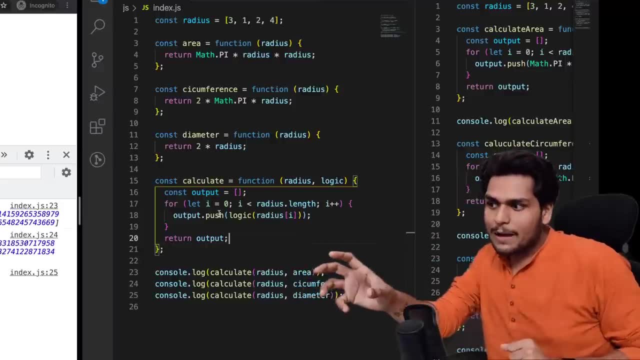 Definitely. If I am your interviewer, I would expect you to write this: Okay, And now let us just see that. why this code is good And this is the beauty of functional programming. I would just tell you in a while. So now, if you see clearly, 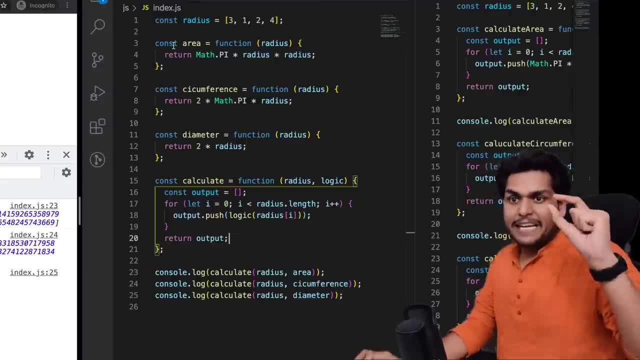 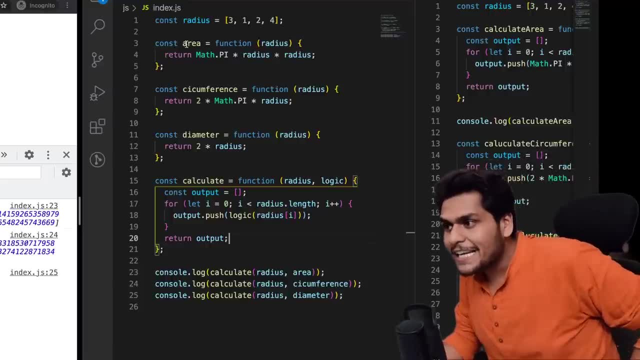 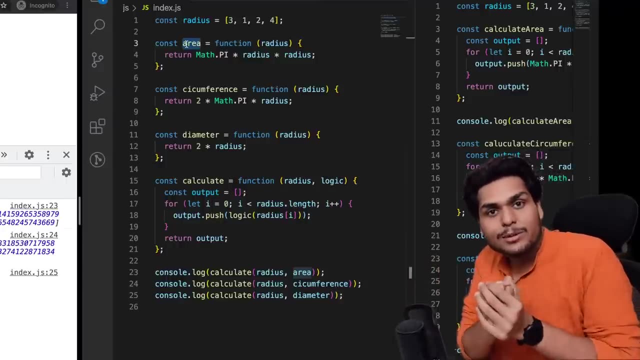 we have abstracted our code into smaller functions and each and the every unit of the function has its own responsibility. If you see this function area, it has just one task to do, that is, calculate the area of function. Circumference is just one task: to calculate circumference. 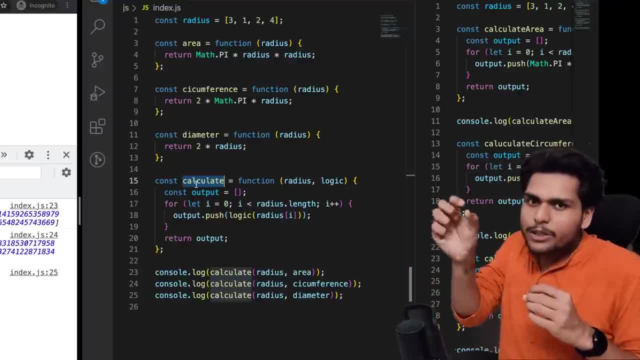 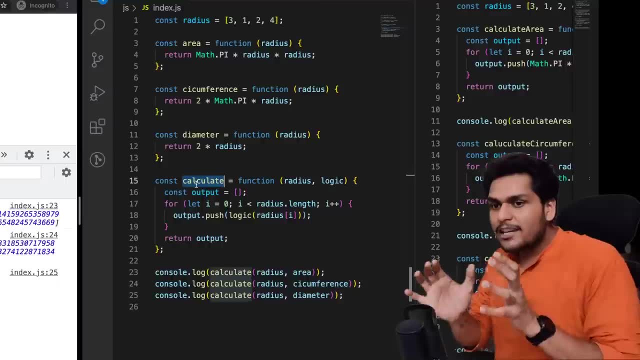 So now this function, calculate, has just one task: to create a new array. I trade through all the elements in that array and just push into the output and return that array. That is the only job Calculate does and we are not repeating anything over here now. 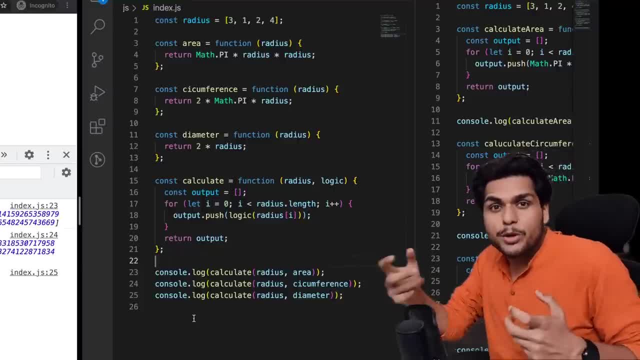 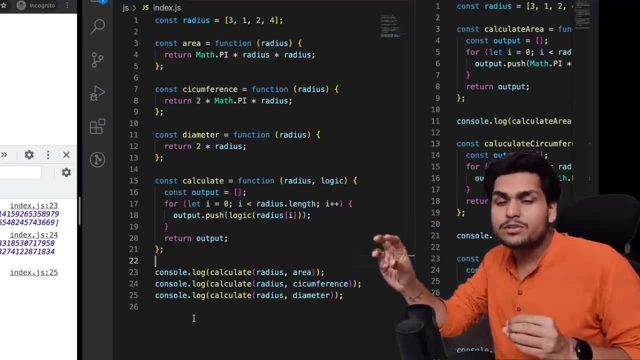 right. So this is the functional programming and this is the beauty of functional programming, where you think everything. they think all the logic into small, reusable components which are functions, Okay do. functional programming is huge in itself and it has a lot of things, but these are crucial things in functional programming: reusability, modularity. 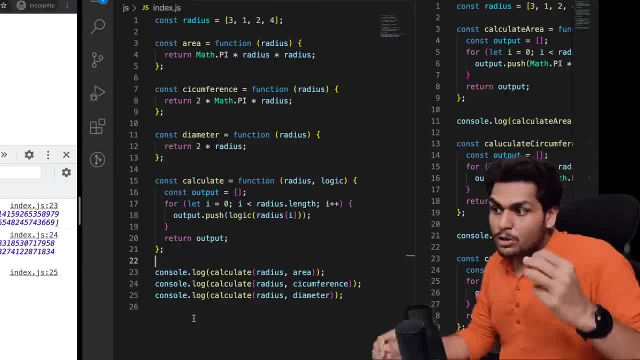 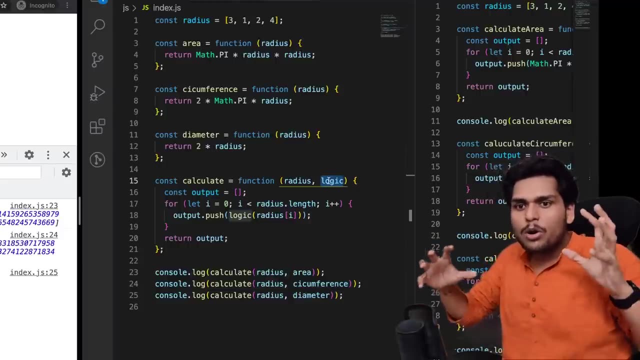 How you pass in functions into different functions. So if you see that now called calculate function is a higher order function, right, and these functions area is a callback function which is passed inside the logic sometimes. so this is how the whole things: callback function, higher order function and everything is merged and this is how you write code. 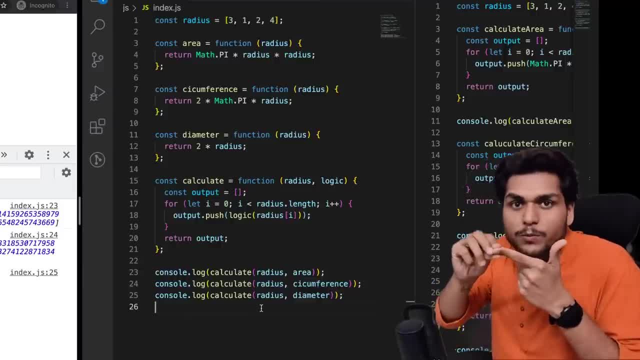 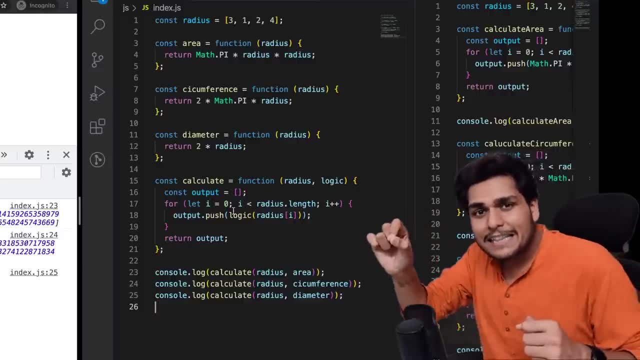 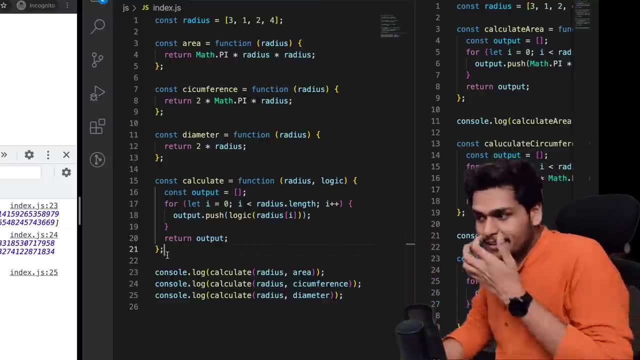 So functional programming deals with pure functions, composition of functions, reusability, modularity and a lot of other things. In the interviews you should be focusing upon writing in this style of code and breaking down your logic into smaller functional units. So now let me tell you something really very interesting. 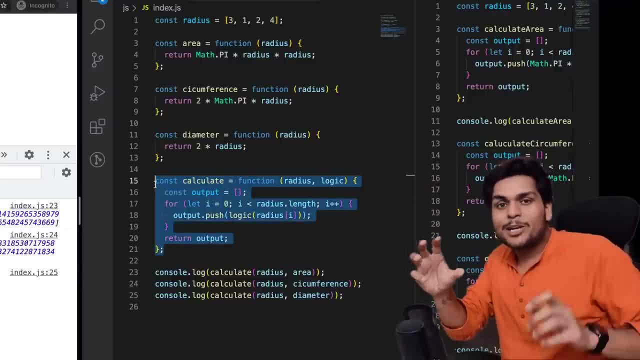 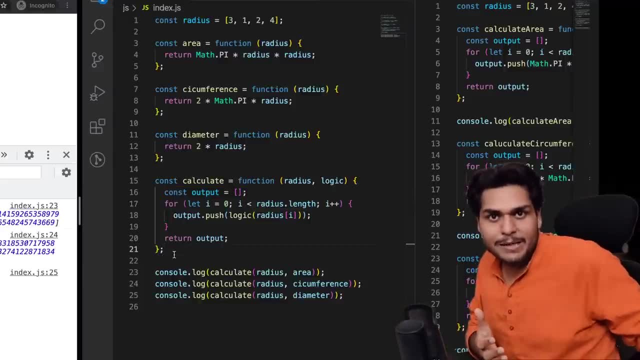 So this function calculate over here is exactly similar to the function map, Isn't it? So if you watch carefully, people who are writing JavaScript for some time now or people who are writing react also might have encountered this function map, where we map a lot of things. map is a very common higher order. 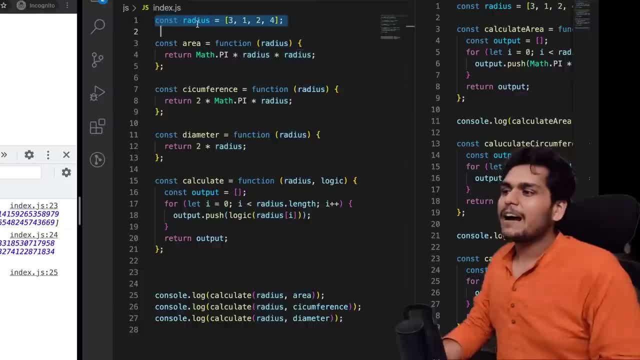 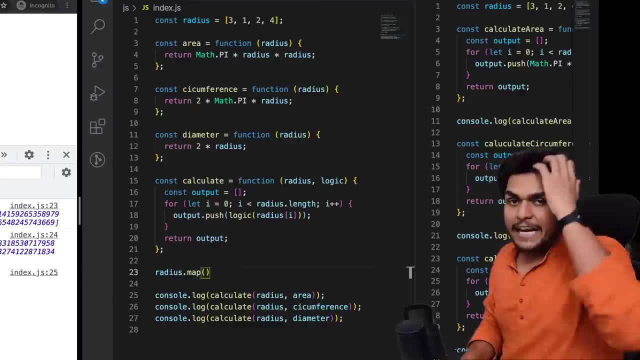 function And how it works. So so if we have this radius over here, if we have this radius array, so there could, there we can write a map function and this map function maps the whole array with some logic. Okay, and that logic is what we pass, suppose if we pass area. 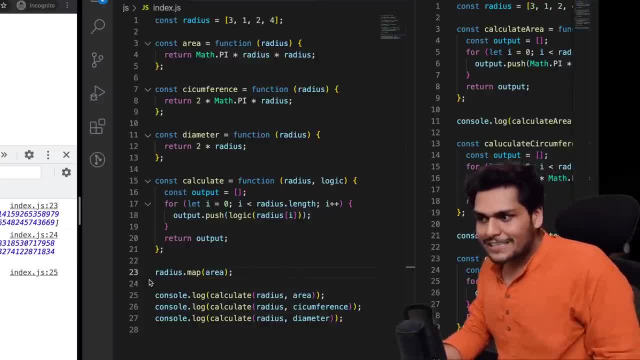 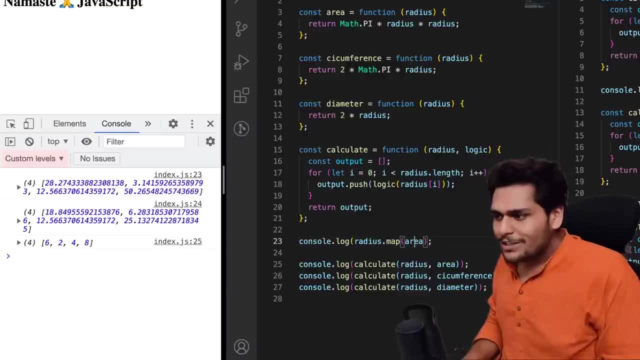 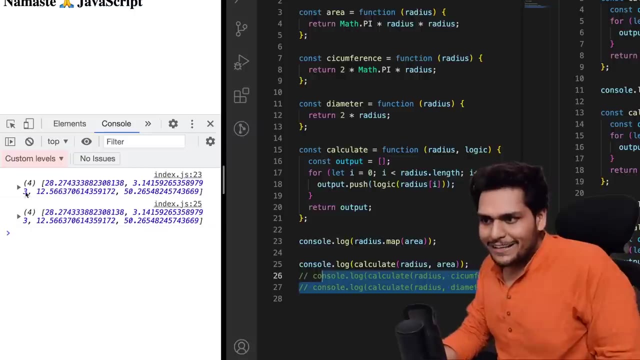 Okay, So this thing will return us an array again and let us see what this array is, Let us just log it. So if you watch carefully- And let me just comment down these two lines- If you just watch carefully, this is exactly similar to map. 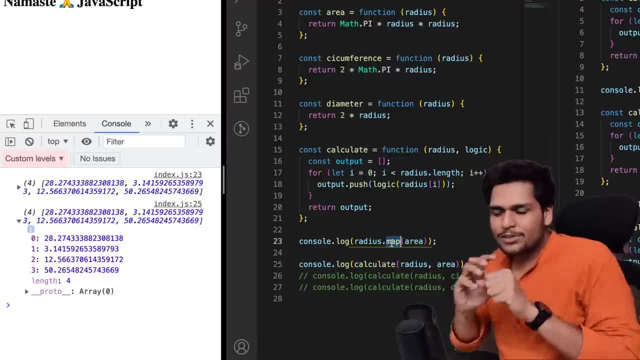 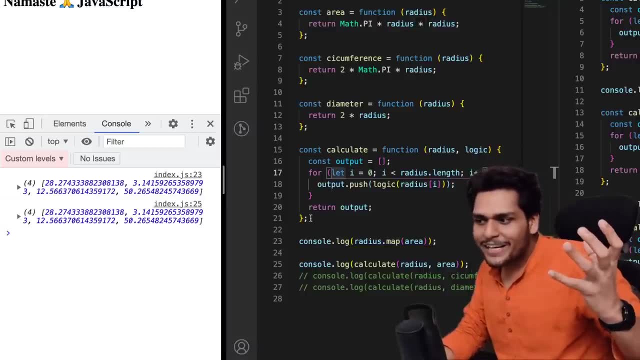 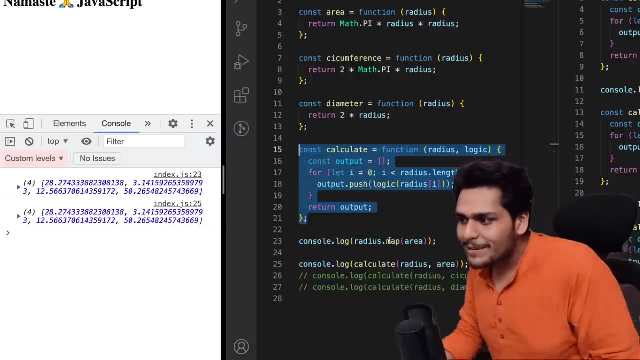 You know this calculate function and map function as almost similar. They are giving us see the same result. So you can say that we kind of wrote our implementation of map over here. We wrote our implementation of map. This map is given by JavaScript to us. 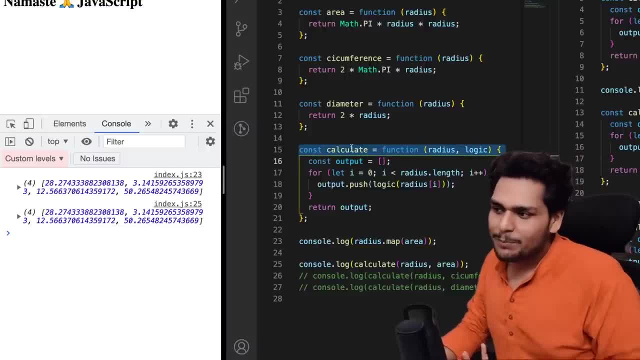 And we have written our implementation of map over here. Okay, obviously like we should rename this radius to ARR or array or something We should make it more generic over here. And this is exactly what map does. What is map doing behind the scenes? 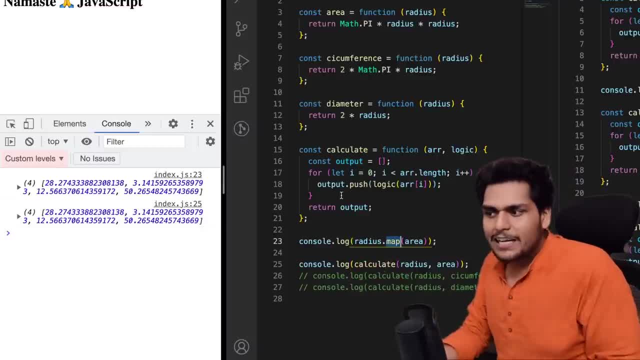 Obviously it would be doing a little more checks, but in a nutshell it is a small implementation of the map function. You know what isn't it interesting? So map function also just creates a new array and then iterate over each of these elements in the radius. 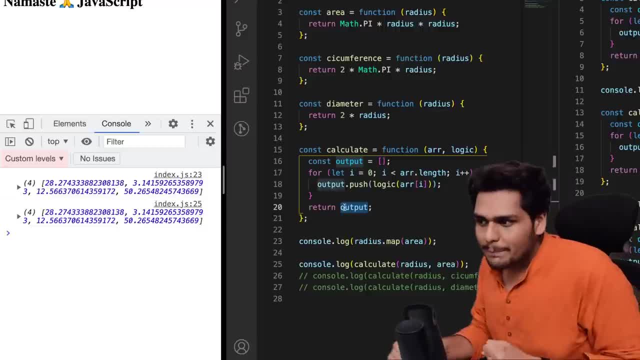 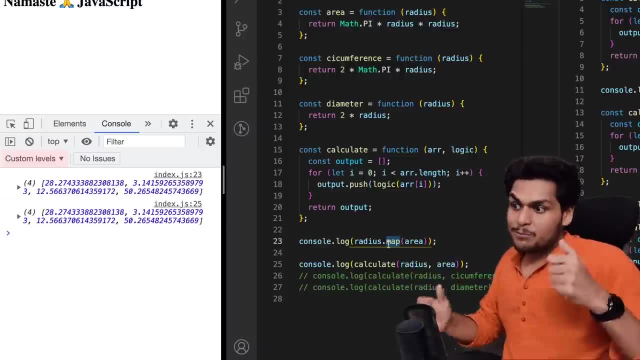 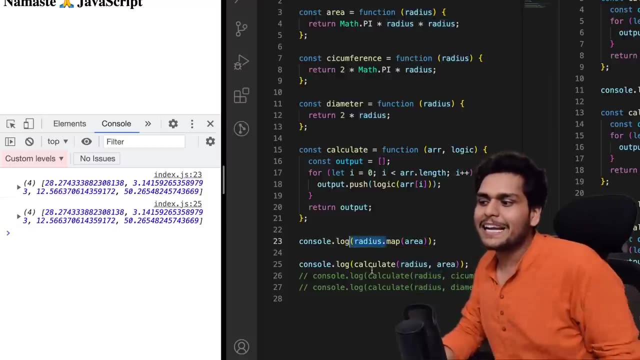 and then returns the output. This is what map is right. What is the difference between our calculate function and map? Nothing, right? It is almost similar. Now you might argue that we are calling this radius as radiusmap and your function is taking radius as an argument. 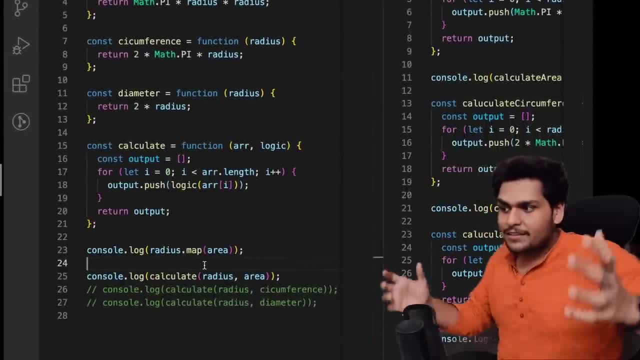 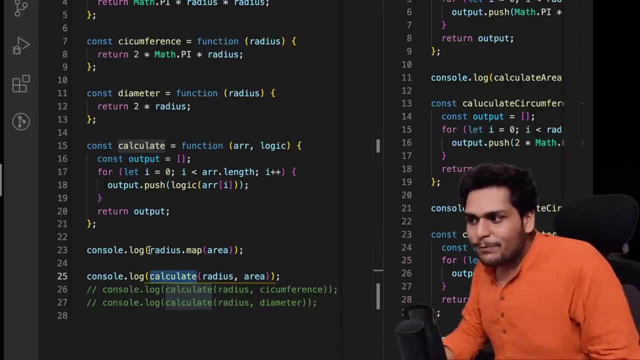 So, but for argument sake, let's try to make this calculate function exactly similar to map. Okay. So when you say exactly similar, if we had to call this function like this, dot map, Okay, array dot map. So what we need to do is we need to do just a small thing. 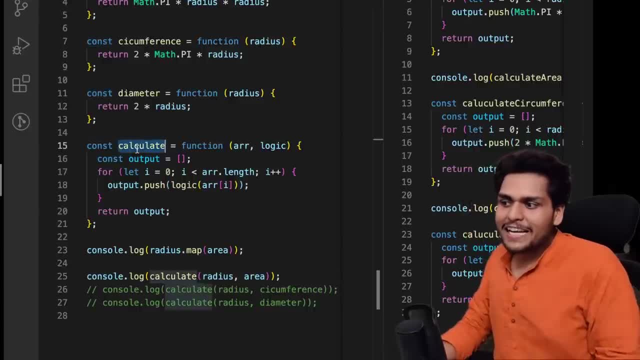 We just need to do. We just need to put this function calculate on the array dot prototype. Okay, you can do like this. I know a lot of people commented last time and told that how can we write functions like that? But this is how you write. 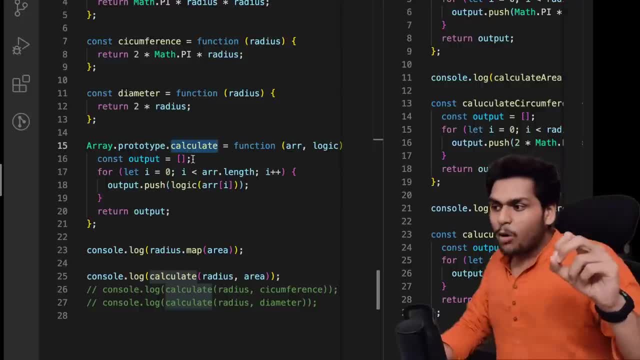 So you can do array dot, prototype dot, calculate. Now this function calculate will be available on all the arrays. you see Okay in your code. So when we put something on to prototype it appears in all the arrays. So that means just like a dot map. 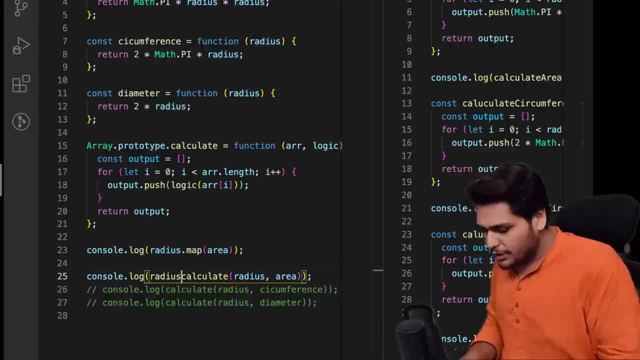 We can also calculate. We can also call radius, dot, calculate now. Okay, this is the power, what we get. Okay, let us try to make it very similar to map. Okay, so this calculate over here takes two arguments, map takes one. 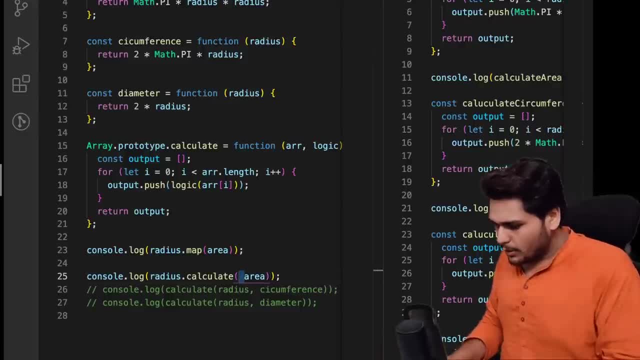 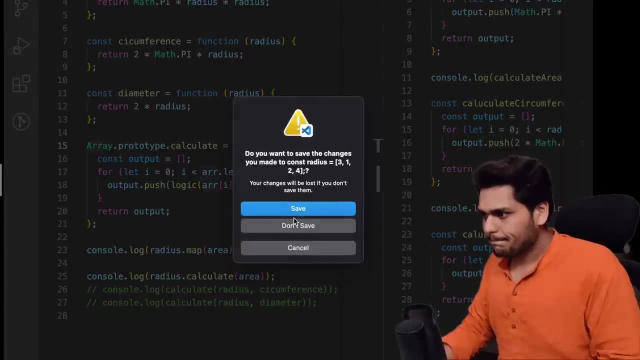 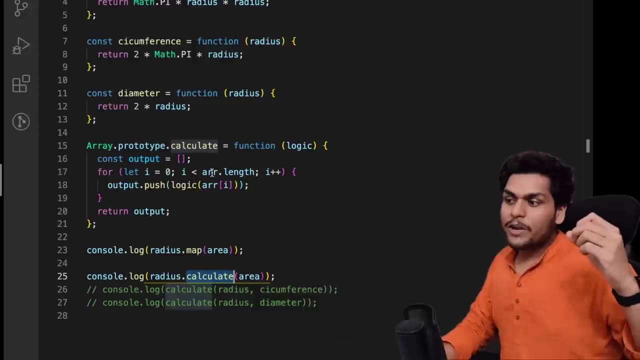 So let us just remove this, for that what we need to do. We need to remove this logic, this ARR also Let me just remove this tab. Don't save so over here. So instead of ARR. So now you would be asking that: where do we get array from? 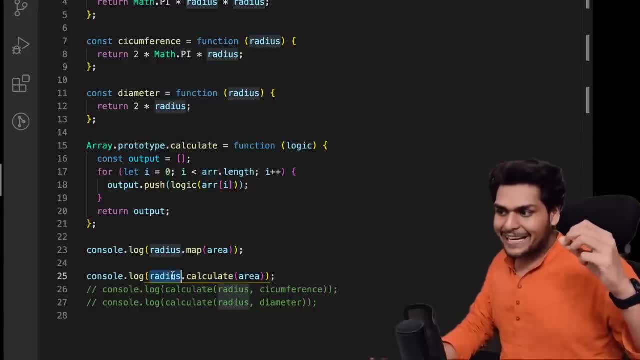 So in this case, when you do a array dot calculate, so over here in the calculate function, that this over here points to the array which is this calculate being called upon. Okay, so I know it might be a little complicated, but see this over here would be the radius. 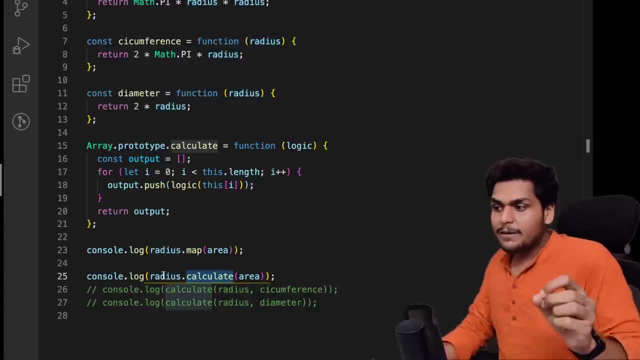 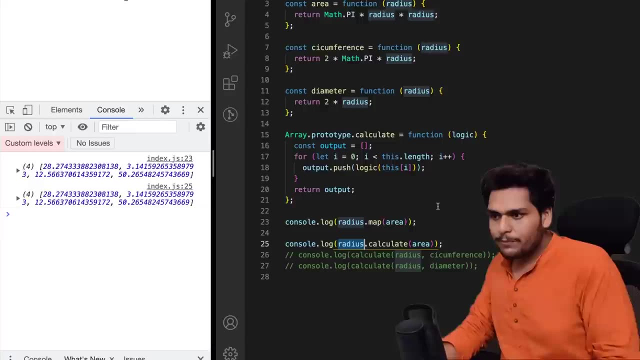 Okay, so when you write radius dot, calculate, so that means that this in the calculate function, which will be pointed to this array. And if I run this code now, if I save it now, see the output. It is exactly same for some people. 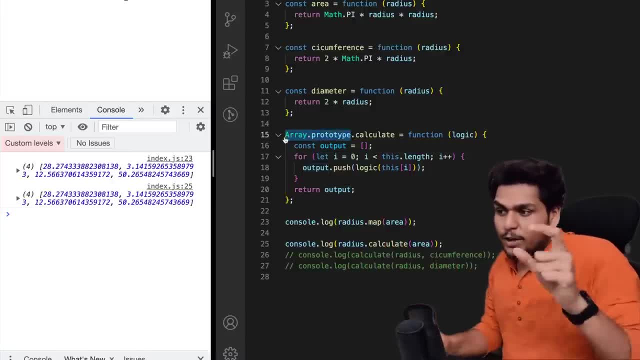 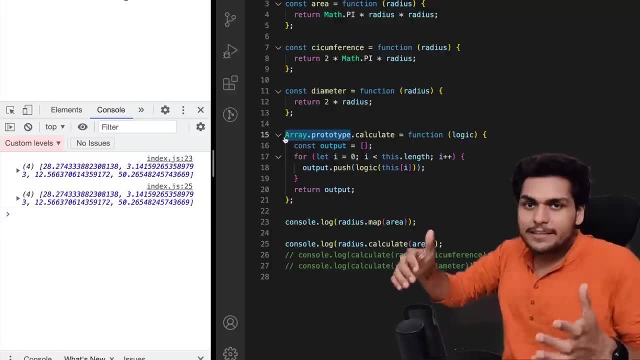 This array dot prototype might have got a little complicated, So I would request you to go and watch my prototype inheritance and prototype video. I link it somewhere in the over here or in the description, but go and watch that video and you will understand it properly. 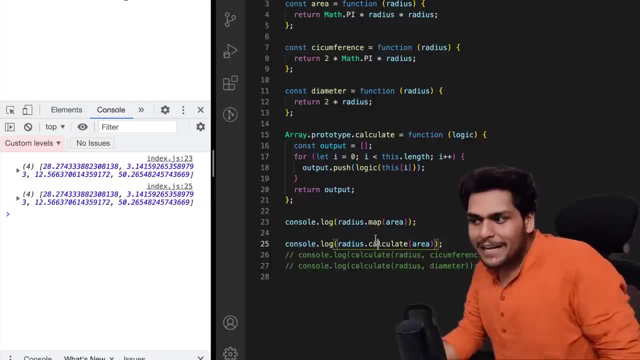 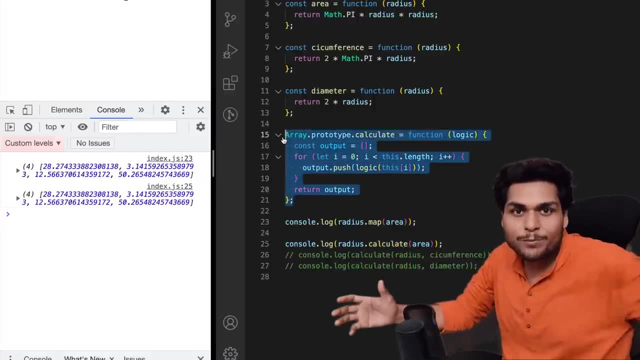 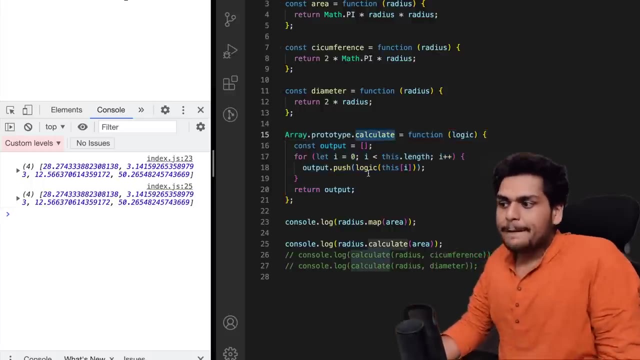 But tell me one thing: Isn't it similar to map? very much similar to map, this map and calculate, isn't it a very small implementation of map? So this is how generally we write the polyfills. So this is kind of like a polyfill for map. 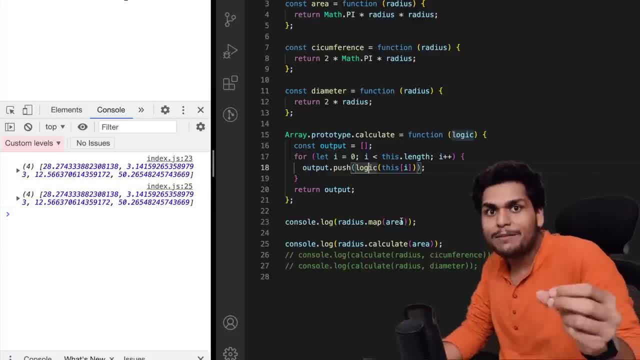 So this is the beauty of functional programming And I hope you have loved this type of code And next time in the interview always try to break down your code into these smaller pieces. This is just an example. It could apply to anything what you are coding. 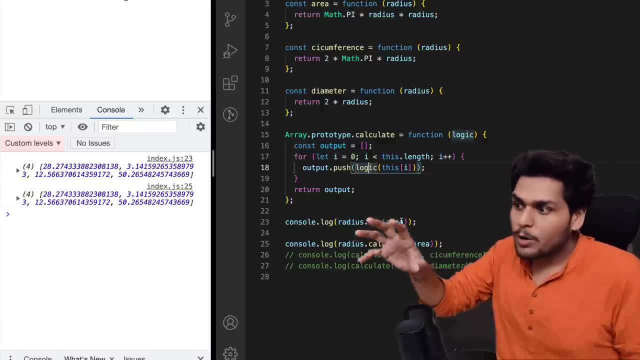 But generally, if I am your interviewer, I am very much careful about how you write code, how modular it is, how reusable it is And how did you think through the logic? This is how you can improve and optimize. So now let's just do a quick recap.